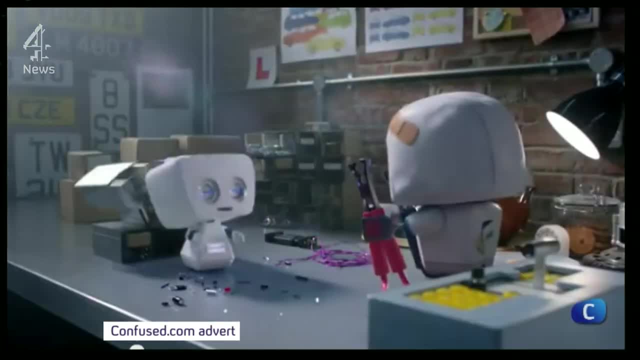 button for savings products. So Confusedcom is just showing consumers like Tony the deals from the eight companies it seems to have already added. So we're not even sure who's going to get them, But we're sure that there are people taking it seriously And we can't. 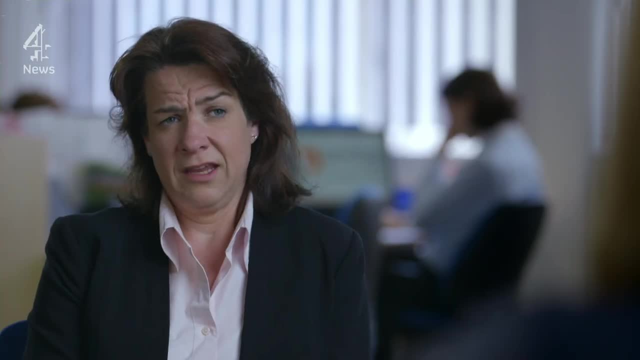 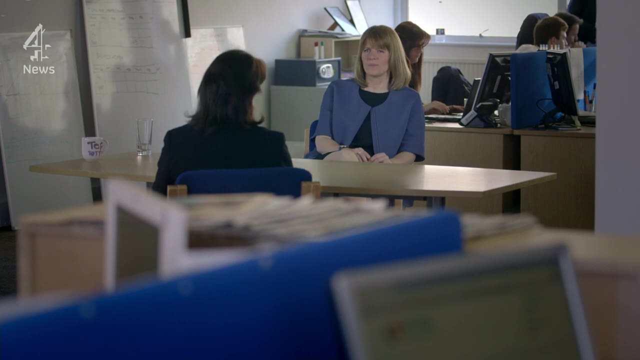 change the market. In our view, the problems that consumers are experiencing are trying to have relationships with. There's a huge disparity in terms of the information and the savings accounts that are monitored by comparison sites. There may be some cases where there are commercial arrangements in place. 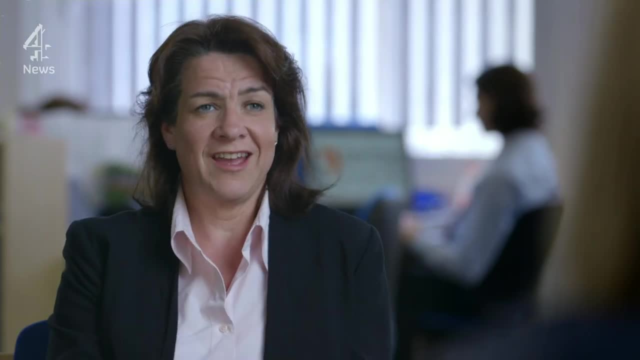 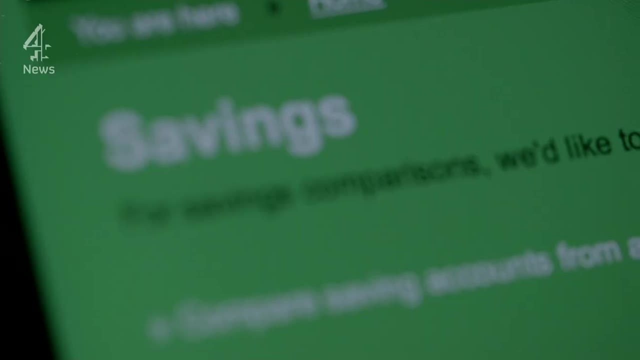 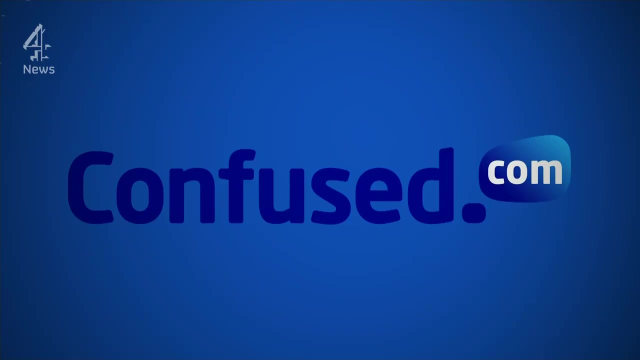 that means that they're promoting the products that earn that comparison site some money, rather than promoting all accounts. It's true that all the other comparison websites have commercial relationships too, But in our investigation, Confusedcom performed the worst by far. In fact, when we approached Confused with our findings, 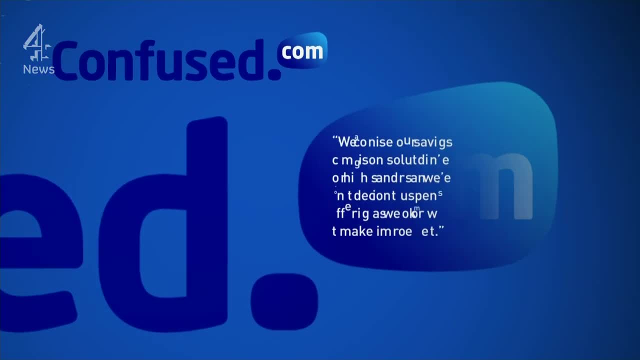 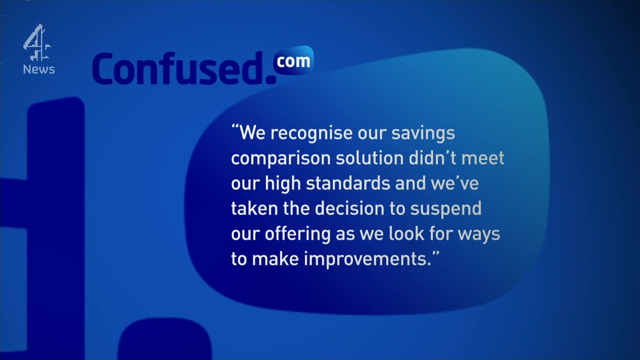 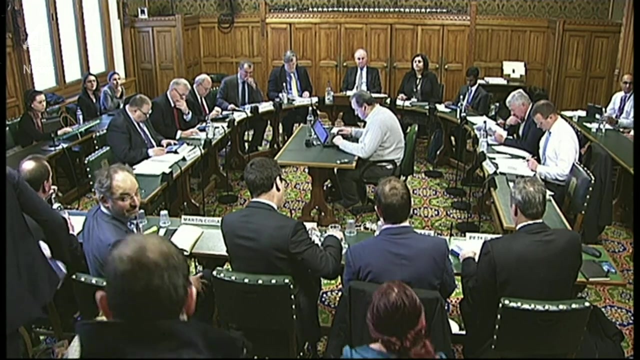 it immediately took down the savings section of its website. It told us We recognise our savings comparison solution didn't meet our high standards and we've taken the decision to suspend our offering as we look for ways to make improvements Earlier this year. the big four comparison websites: 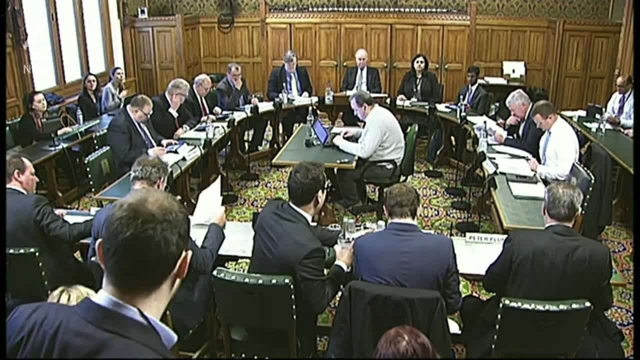 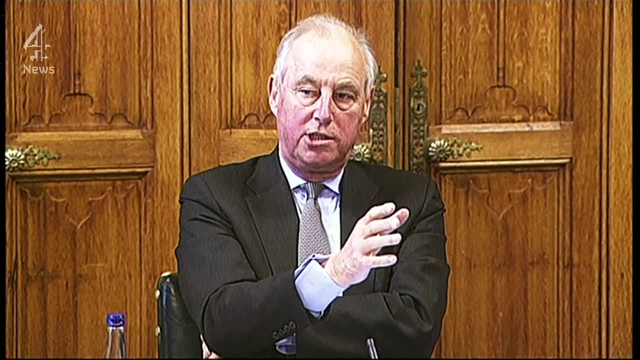 were hauled in front of politicians to answer claims about their recommendations in the energy sector, And last week Ofgem, the energy regulator, said it had launched an investigation into whether they have breached competition law. So you might think someone would be keen to step in now. 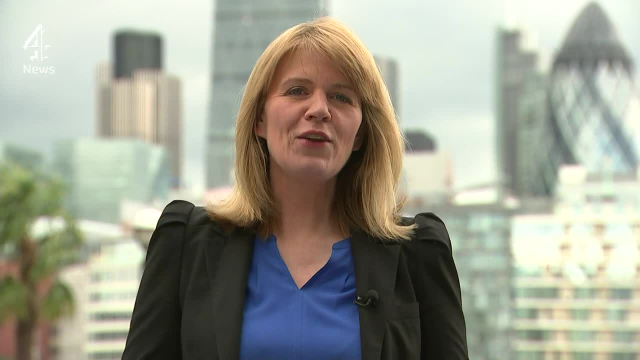 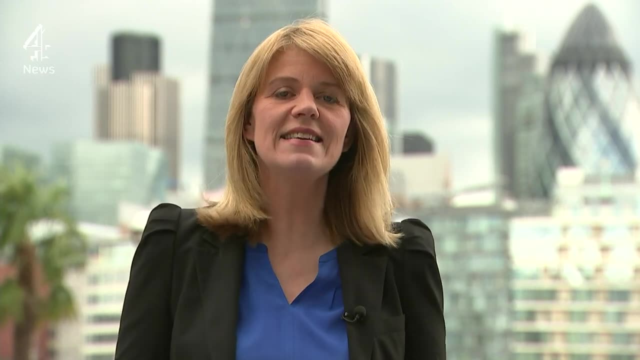 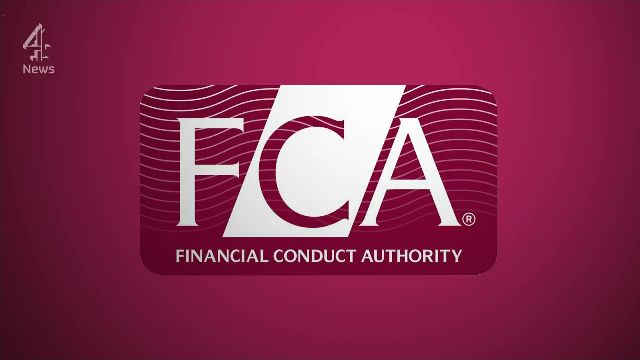 and investigate Confused's admission. But Channel 4 News has learned there is no-one to step in and investigate since the FCA, the regulator, has conceded there's no-one regulating these activities anyway on the comparison websites. But what the FCA did tell us. 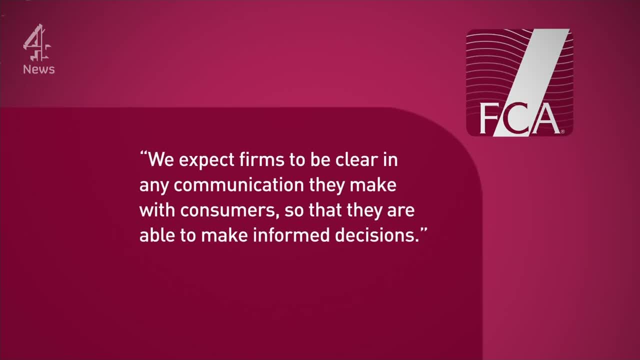 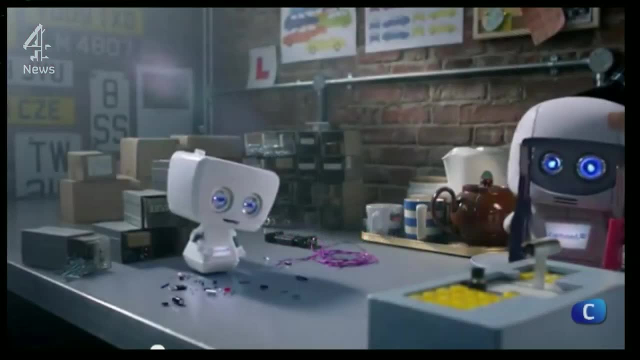 was that we expect firms to be clear in any communication they make with consumers so that they are able to make informed decisions. Tonight, though, the Treasury appeared to signal a tougher line, telling Channel 4 News it stood ready to assist the FCA. 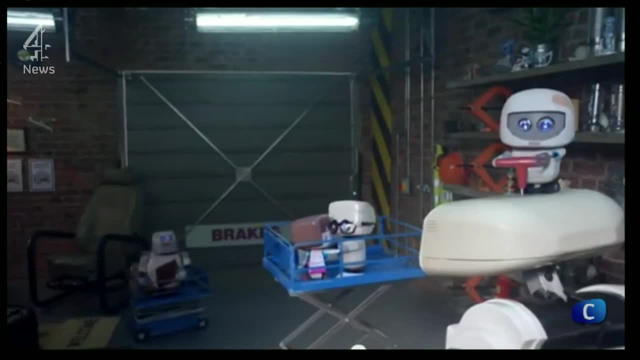 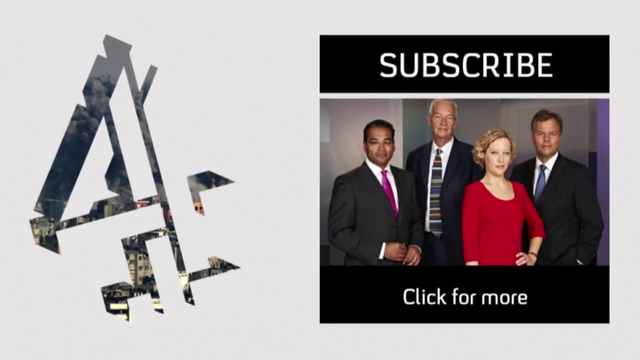 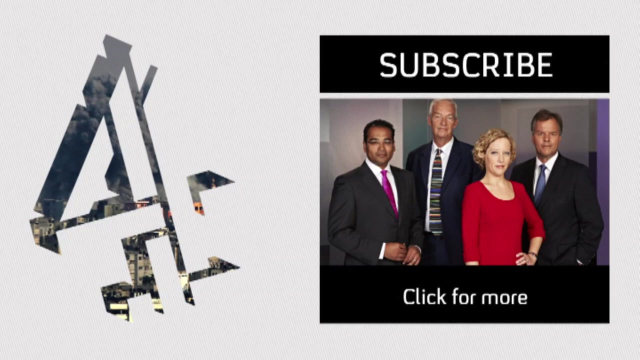 in any probe into the role of price comparison websites in selling us all financial services. Online Mail- Ohhh. Every minute of the week, every day, every minute, an anonymous T-shirt and SMS is wine or pasta or a steak or La Crosse. A Roman Monsoon, A top or a melhor. Hello, Mike, It's me, Mike Bustanko, and I'm an avid cashier from United livestock business.